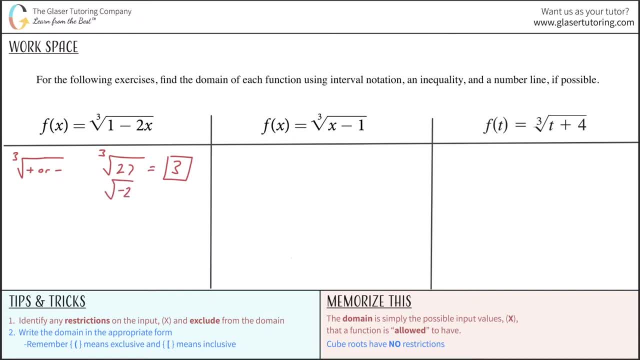 I can take the cube root of negative 27,. okay, Because I'm asking myself what number times itself three times would give me negative 27? And that answer is negative three. now, all right, So you can take the cube root of a negative number unlike a square. 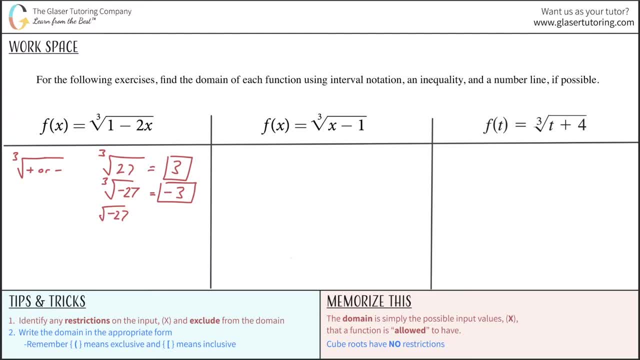 root. You cannot take the square root of 27.. It's impossible, all right. No number times itself will give you a negative number, all right. So, that being the case, we realize the why now that cube roots have no restrictions. 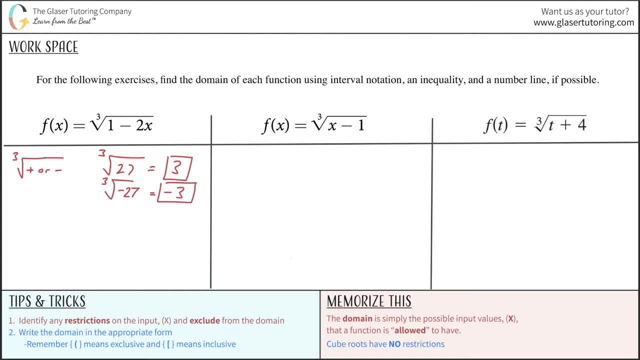 Basically. so now we can begin to develop our notations. all right, No restriction, meaning it can go all the way from negative infinity, meaning the x value all the way from negative infinity to positive infinity. So now, that being the case, right, our interval notation will be simply from: 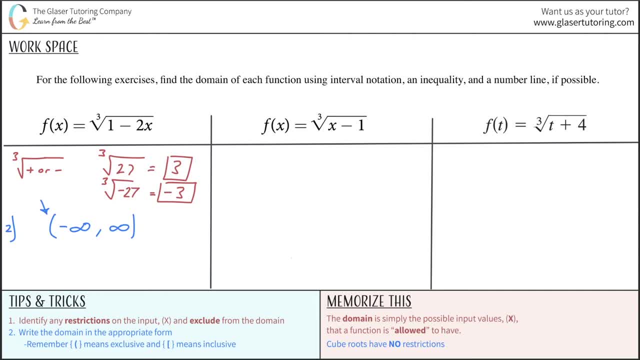 negative infinity. comma positive infinity. These parentheses mean exclusive of the value. You can never include infinity. okay, It's an idea, not a real number. So we're going to take the cube root of a negative number. So this is the interval notation In terms of the inequality, once you have the interval. 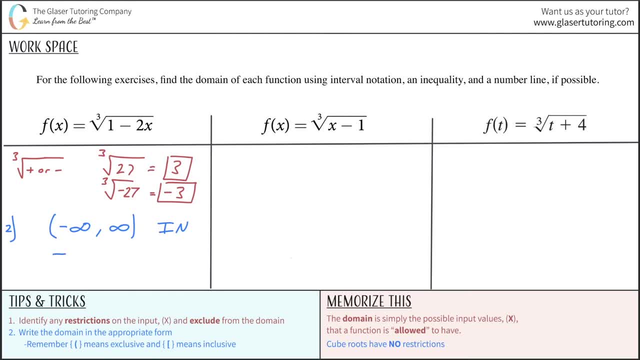 notation here. it's simple: Just plug in your x in the middle, meaning that it can go from negative infinity and that will be less than x, and then x will be less than infinity. right, This is your inequality. now okay for the domain, all right. And then, last but not least, we can create now our 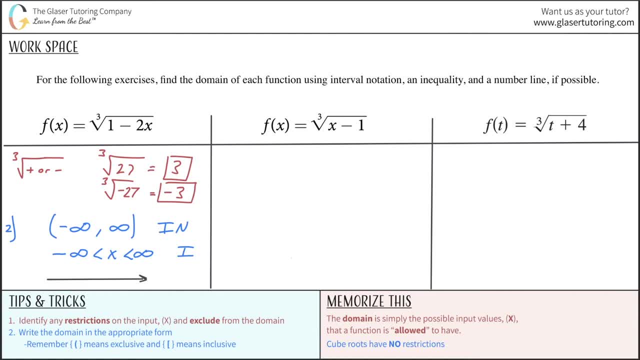 number line and if we create our number line right we draw a lot of arrows here. Here's the value of zero Negative infinity out there all the way to positive infinity on the right, and we realize that it's all real numbers and it includes negative infinity, not includes, excuse me, it excludes. but 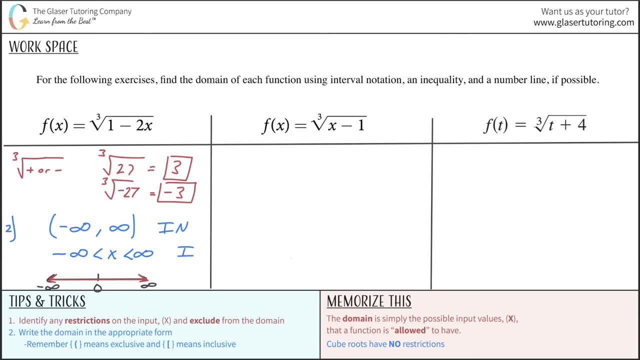 it goes all the way out to negative infinity, to positive infinity. all right. So now taking a look at the next one. let's see if we can run through this, All right. so the next one. look, we're taking a cube root, okay, And remember, there's no restrictions, There's nothing else going on here. 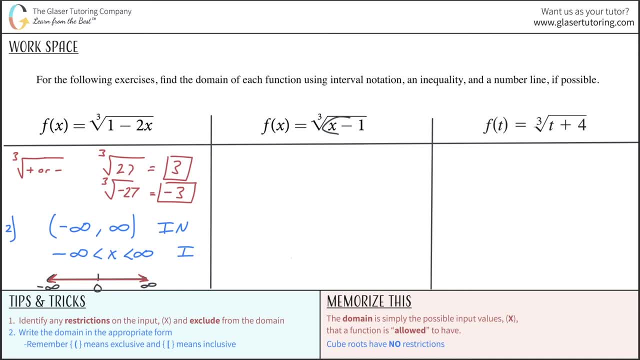 X can be whatever number I want It can be. uh, because the total here can be a negative value or a positive value, right? So there are no restrictions and therefore the answer is literally the same as we found over here. So all I'm gonna do is: